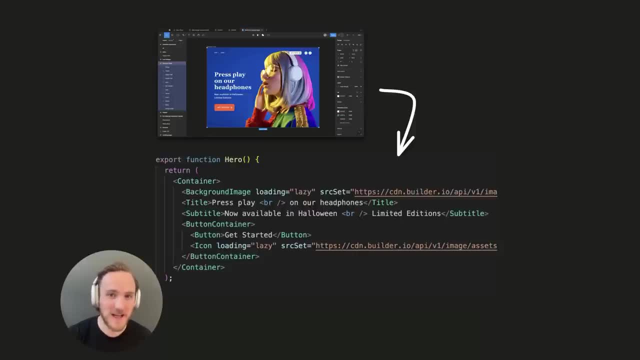 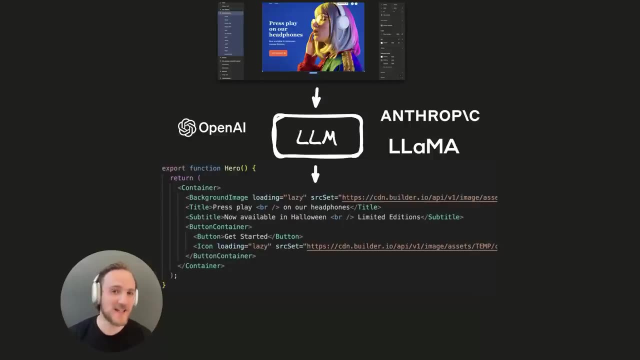 smaller pieces. You need to break down your problem into smaller pieces, And you need to In our case. we wanted to take any Figma design and automatically convert that into high-quality code. In order to break this problem down, we first explored our options. The first one, I'd 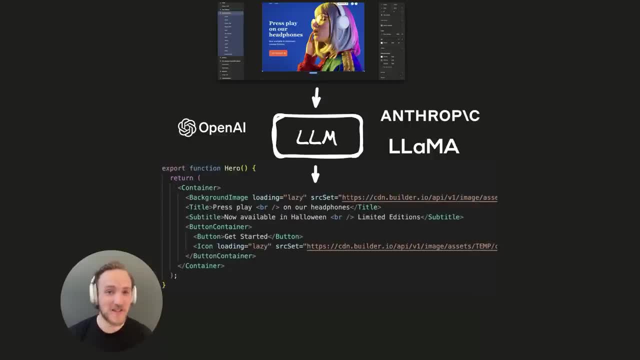 suggest you always try is basically what I suggested not to do, which is see if you can solve your problem with a pre-existing model. If you find this effective, it can allow you to get a product to market faster and test on real users, as well as understand how easy to replicate this. 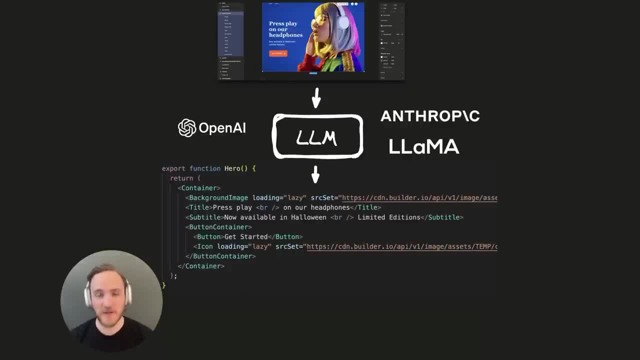 might be for competitors And ultimately, if you find this works well for you but some of those drawbacks I mentioned become a problem, you can try it out And if you find this works well for such as cost, speed or customization, you could train your own model on the side and keep. 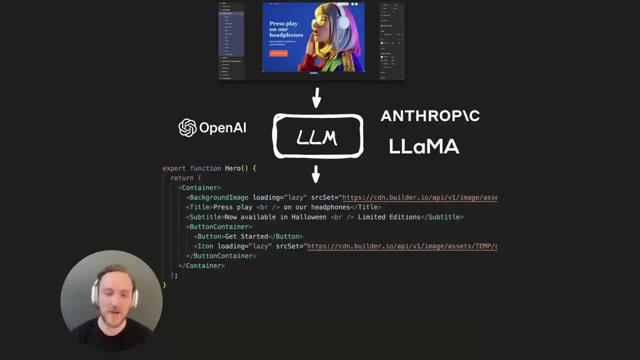 refining it until it outperforms the LLM you tried first, But in many cases you might find that these popular general-purpose models just don't work well for your use case at all. In our case we tried feeding it Figma designs as raw JSON data and asking for React components out the other side. 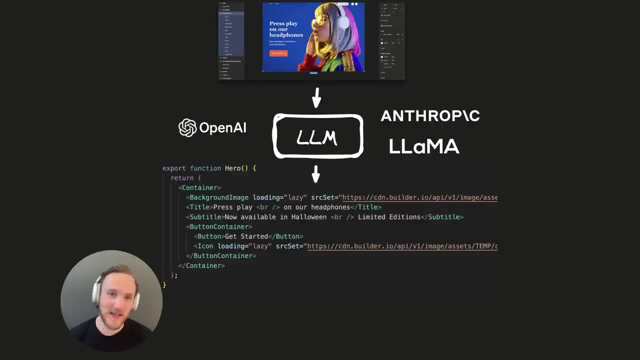 and it just frankly did awful. We also tried GPT-4V and taking screenshots of Figma designs and getting code out the other side And similarly, the results were highly unpredictable and often terribly bad. So if you can't just pick up and use a model off the shelf, 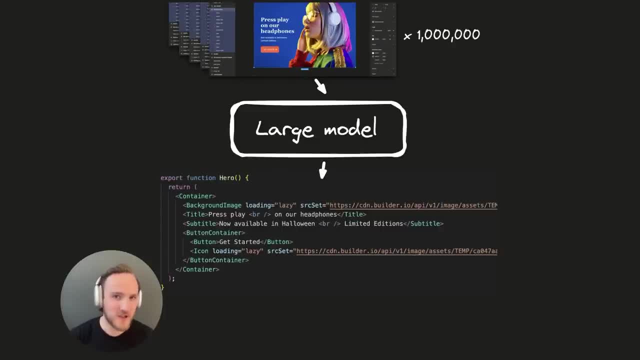 now we need to explore what it would look like to train our own. A lot of people have the intuition. let's just make one big giant model where the input is the Figma design and the output is the fully finished code. We'll just apply millions of Figma designs with millions of code snippets. 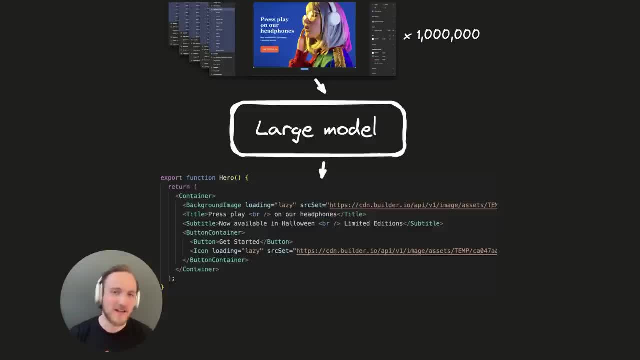 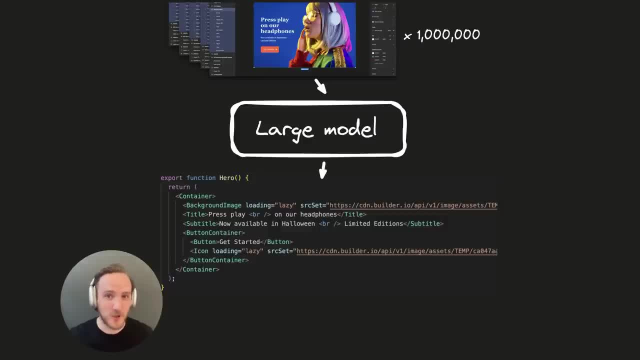 the more costly it is to train. Large models also take a lot of time to train, So as you iterate and make improvements, your iteration cycles can be days at a time waiting for training to complete. And even if you could afford that amount of time expense and have the expertise needed to make, 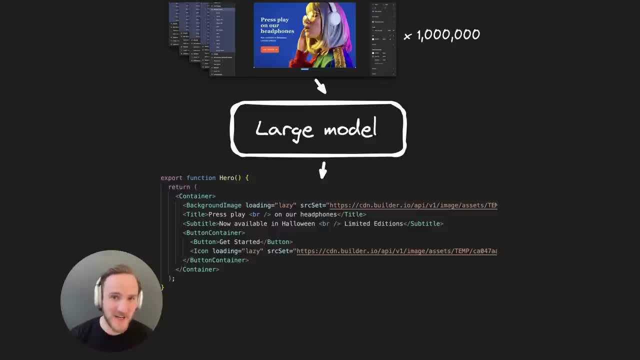 these large, complicated custom models, you may not have any way to generate all that data you need anyway. If you can't find this data on the open web, then are you really going to pay thousands of developers to hand code millions of Figma designs into React? 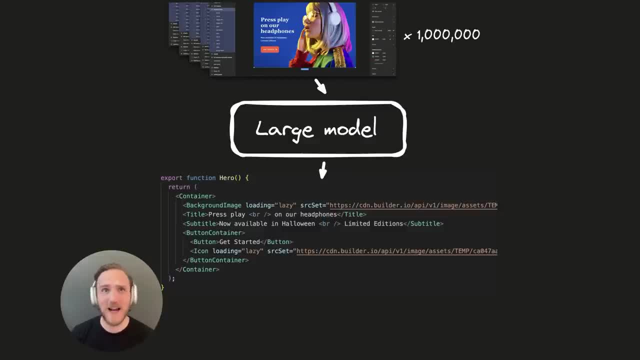 Or any other framework, let alone all the different styling options like Tailwind versus Emotion versus CSS modules, It just becomes an impossibly complex problem to solve, And a super duper model that just does everything for us is probably not the right approach, here At least. 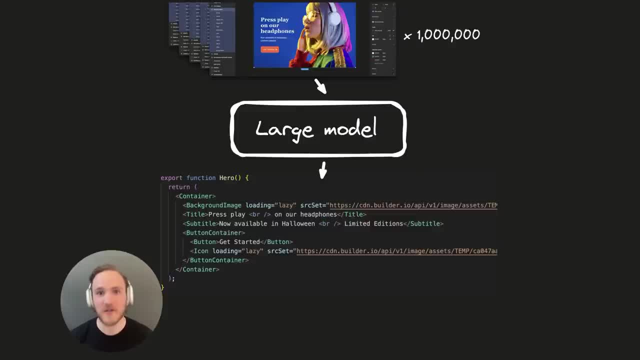 not today. When you run into problems like this, I would highly recommend trying to swing the pendulum to the complete other end and try as hard as you can to solve as much of this problem as possible without AI whatsoever. That forces you to break the problem down into lots of discrete. 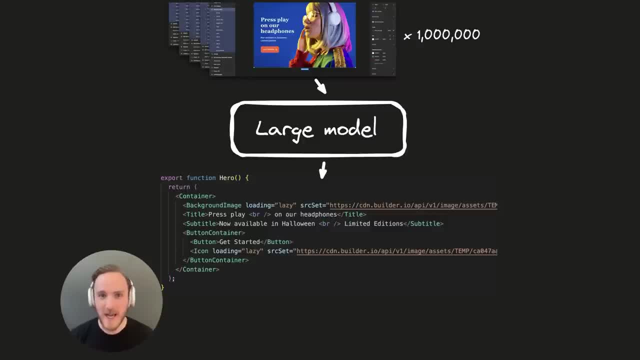 pieces that you can write normal traditional code for and see how far you can solve this. In my experience, however far you think you can solve it with some iteration and creativity, you can get a lot farther than you think. When we tried to break this problem down into just 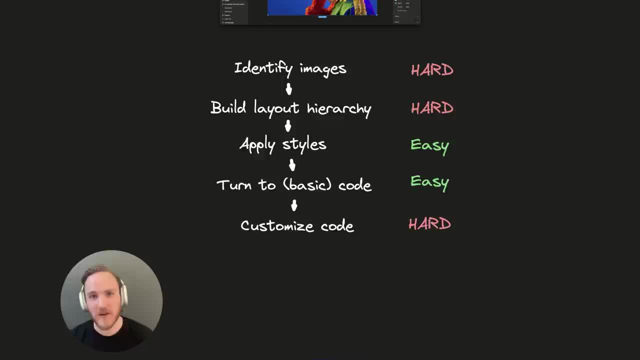 plain code, we realized that there were a few different specific problems we had to solve. In our findings, at least two of the five problems were really easy to just solve with code. Where we hit challenges was in those other three areas. So let's take that first step of identifying images. 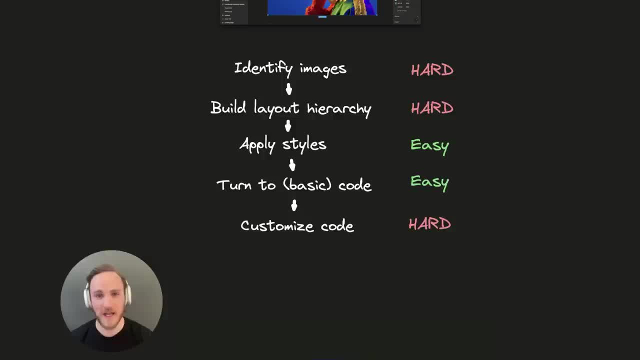 and cover how we can solve this problem. Now we can train our own specialized model to solve this use case. You really only need two key things to train your own model these days. First is identify the right type of model And second, you need to generate lots of example data. In our case, we're able to find a very common type. 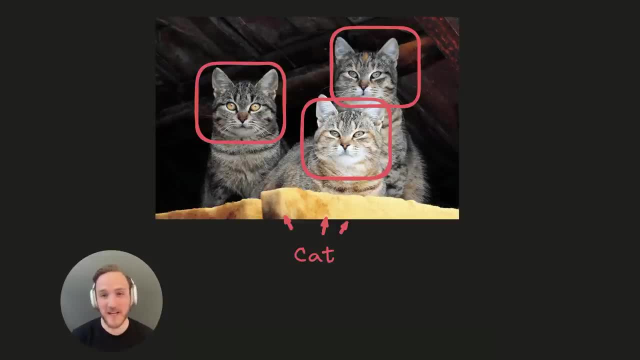 of model that people train is an object detection model which can take an image and return some bounding boxes on where it found specific types of objects, In this case locating the three cats- And so we asked ourselves: could we train this on a slightly novel use case? 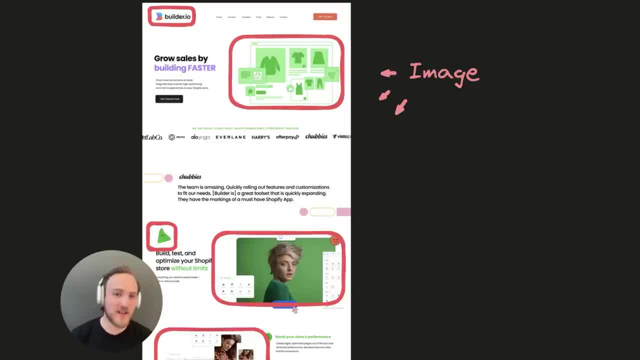 which is to take a Figma design as an image which uses hundreds of vectors throughout. but for a website or mobile app, certain groups of those should really be compressed into one single image and can identify where those image points would be. So we can compress those into one. 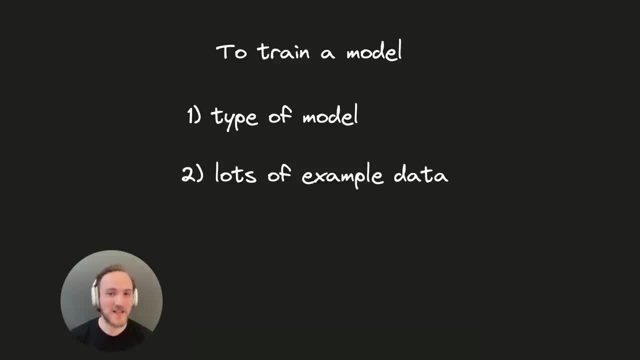 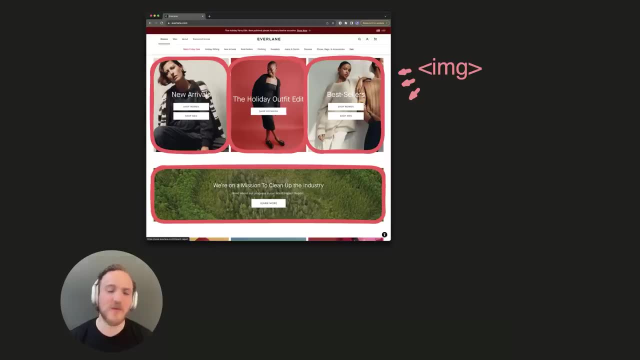 and generate the code accordingly. So that leads us to step two. We need to generate lots of example data and see if training this model accordingly will work out for our use case. So we thought, wait a second, could we derive this data from somewhere? somewhere that's public and free? 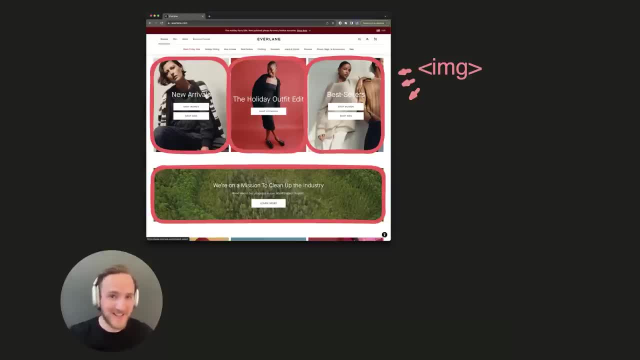 Just like tools like OpenAI did, where they crawl through tons of public data on the web and GitHub and use that as the basis of their training. Ultimately, we realized: yes, we wrote a simple crawler that uses a headless browser to pull up a website into it and then evaluate some. 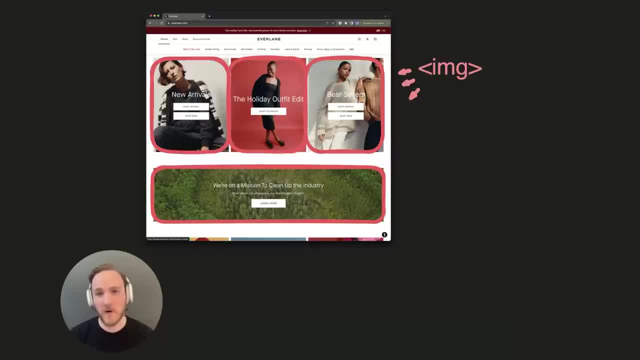 JavaScript on the page to identify where the images are and what their bounding boxes are, which was able to generate a lot of training data for us really quickly. Now keep in mind one critical thing: Quality of your model is entirely dependent on the quality of your data. So out of 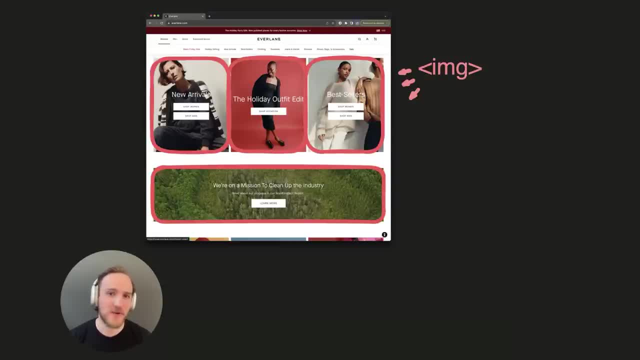 hundreds of examples we generated. we manually went through and used engineers to verify that every single bounding box was correct every time, and used a visual tool to correct it anytime there weren't. In my experience, this could become one of the most complex areas of machine learning. 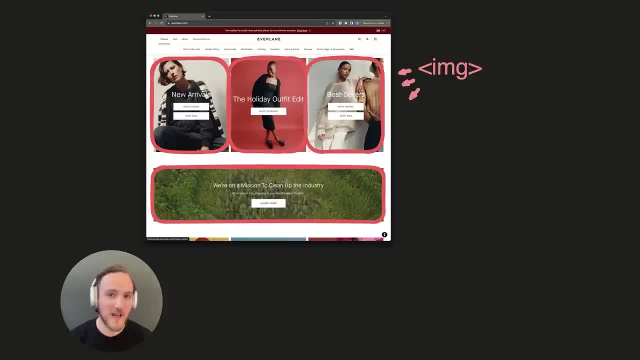 which is building your own tools to generate, QA and fix data to ensure that your data set is as immaculate as possible so that your model has the highest quality information to go off of. Now, in the case of this object detection model, luckily, 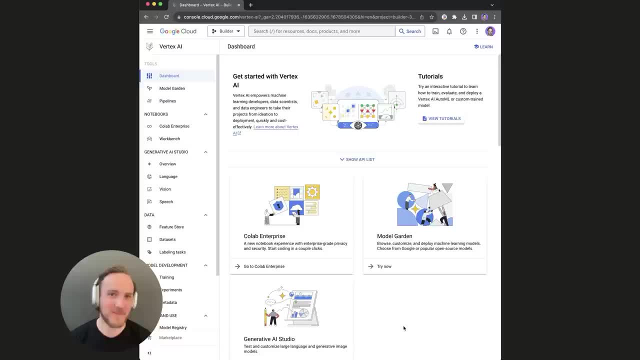 Google's Vertex AI, which has that exact tooling built in. In fact, Vertex AI is how we uploaded all of that data and trained the model, without even needing to do that in code at all. All you need to do is go to the Vertex AI section of the Google Cloud console, go to datasets and hit. 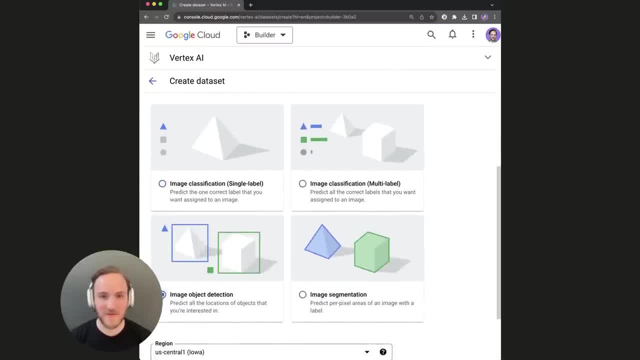 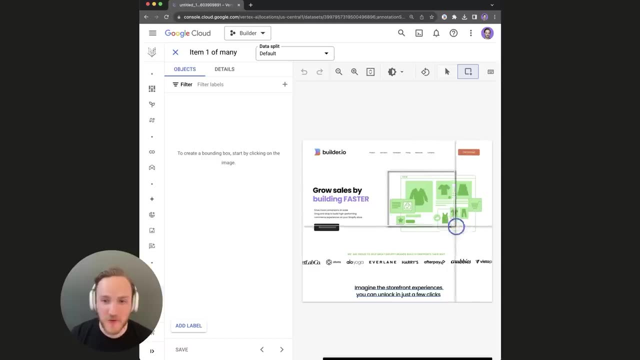 create. We then can choose that we're using an object detection model and hit create, And now you just need to upload your data. You can do it manually by selecting files from your computer and then use their visual tool to outline the areas that matter to us, which is a huge help. 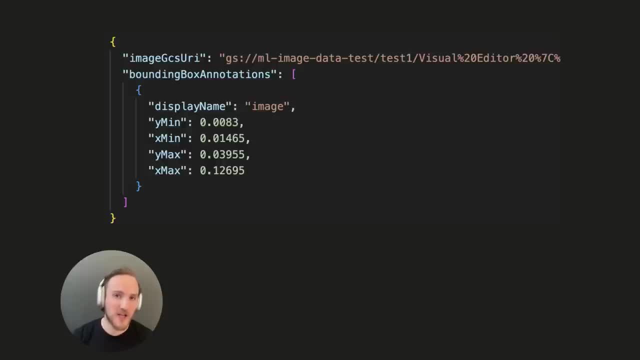 that we don't have to do every day. So if you're using a virtual tool, you can use a virtual tool to do that. You don't have to build that ourselves Or, in our case, because we generated all of our data programmatically. we can just upload it to Google Cloud in this format, where 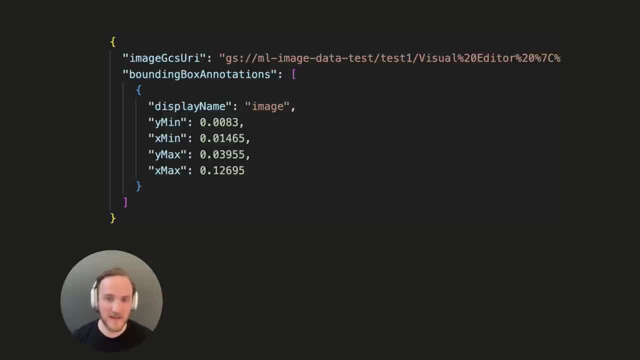 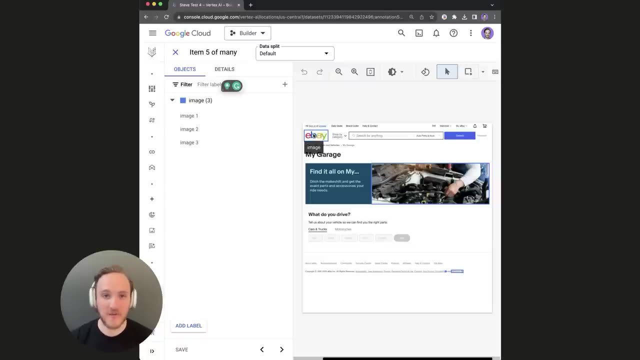 you provide a path to an image and then list out the bounding boxes of the objects you want to identify. Then, back in Google Cloud, you can manually verify or tweak your data as much as you need And then, once your data set's in shape, all we need to do is train our model. I use all 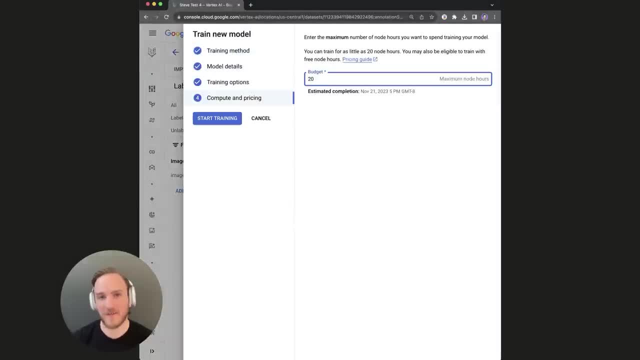 the default settings here and I use the minimum amount of training hours. This is the one piece that will cost you some money. In this case, I'm going to use the minimum amount of training hours. In this case, the minimum amount of training needed costs about $60.. Now, that's a lot cheaper. 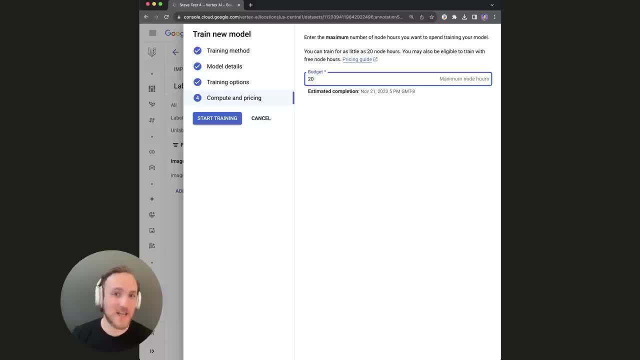 than buying your own GPU and letting it run for hours or days at a time. But if you don't want to pay a cloud provider, training on your own machine is still an option. There's a lot of nice Python libraries that are not complicated to learn where you can do this too, Once you hit. 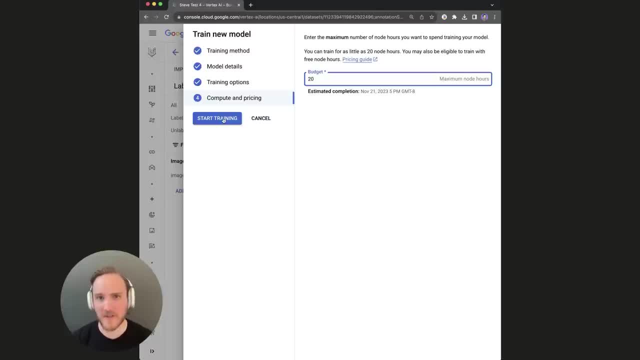 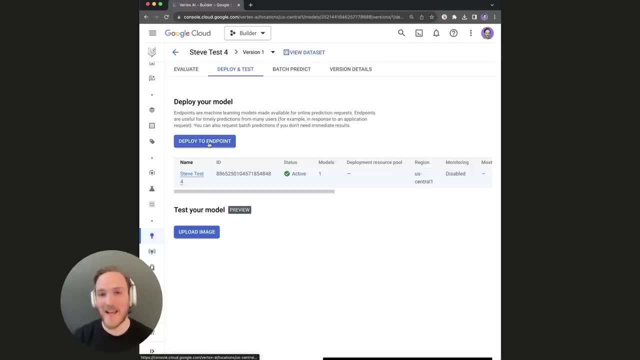 start training- and, in our case, took about three real world hours- then you can find your training results and deploy your model, which in this case I've already done. That can take a couple of minutes and then you'll have an easy way to train your model. So if you're using a virtual tool, 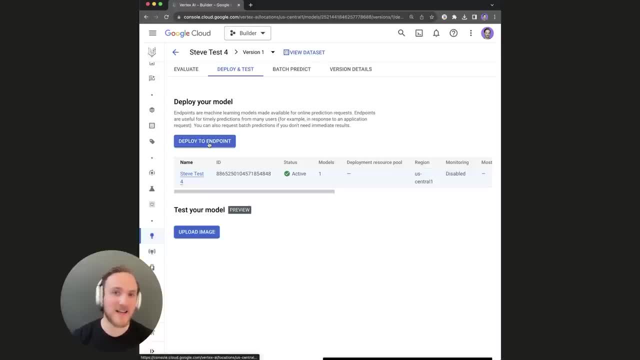 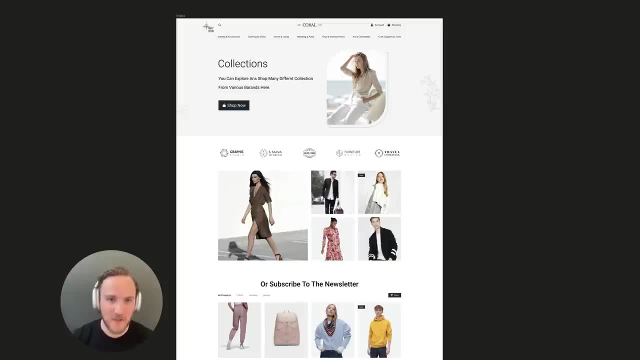 you can also use the API endpoints that you can send an image and get back a set of bounding boxes with their confidence levels. We could also use the UI here as well. So to test it out now in Figma. I'm just going to take a screen grab of a portion of this Figma file because I'm lazy. 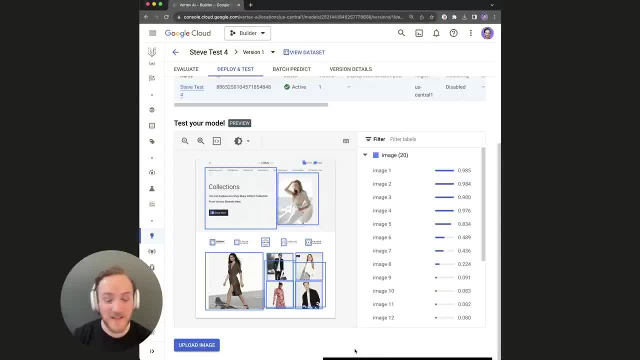 and I can just upload it to the UI to test. And there we go. We could see it did a decent job, but there are some mistakes here. But there's something important to know: This UI is showing all possible images regardless of confidence When I take my cursor. 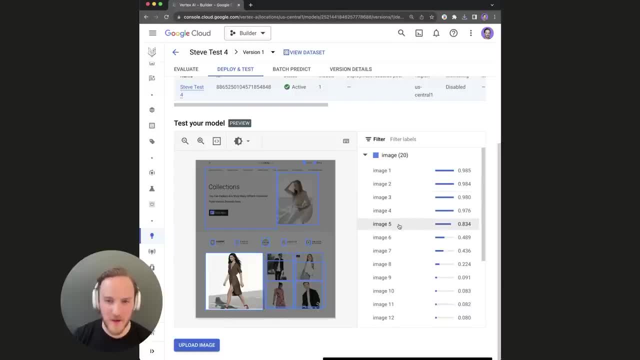 and I hover over each area that has high confidence. these are spot on, These are perfect. Look at that. And the strange ones are the ones down here with really low confidence. I mean, these are just wrong, But that works as expected. This even gives you an API where you 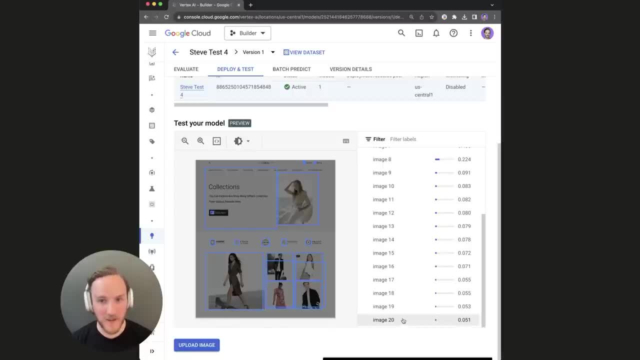 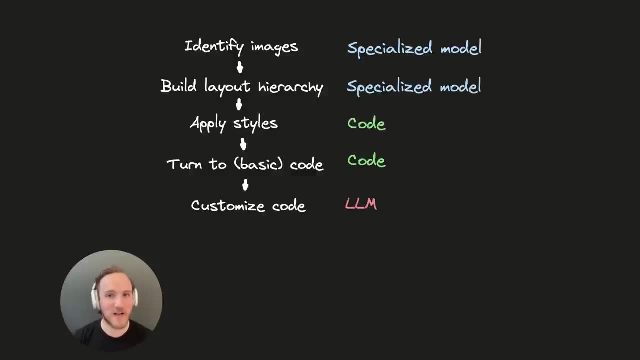 can specify only return results above a certain confidence threshold. By looking at this, I think we want a threshold of at least 0.2.. And there you have it. With a specialized model we can run it wildly faster and cheaper. And when we broke down our problem we found for image identification. 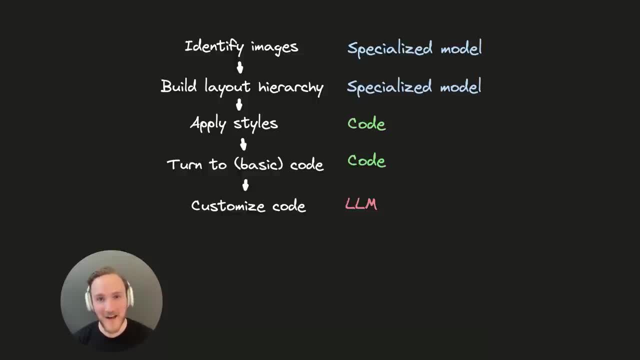 a specialized model was a much better solution For building the layout hierarchy. similarly, we made our own specialized model for that too. For styles and basic code generation, plain code was a perfect solution, And don't forget, plain code is always the fastest. 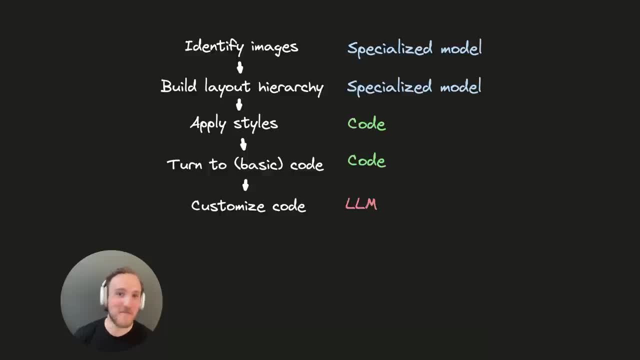 the cheapest, the easiest to test, the easiest to debug, the most predictable and just the best thing. So, whenever you can use it, absolutely just do that. And then, finally, to allow people to customize their code name, it better use different libraries than we already.